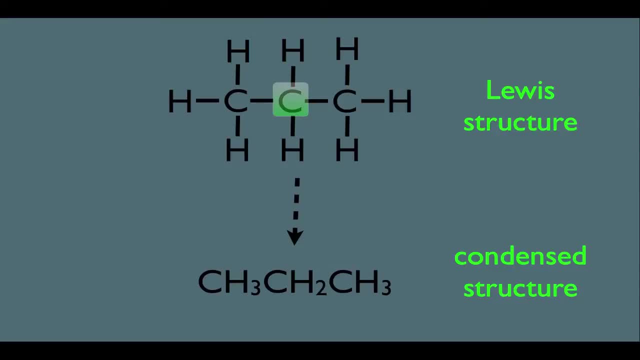 representation: this one right here, this carbon right here, would be this carbon here and the two hydrogens attached to him would be these two hydrogens down here. And lastly, for this carbon over here, would be this carbon down here: His. 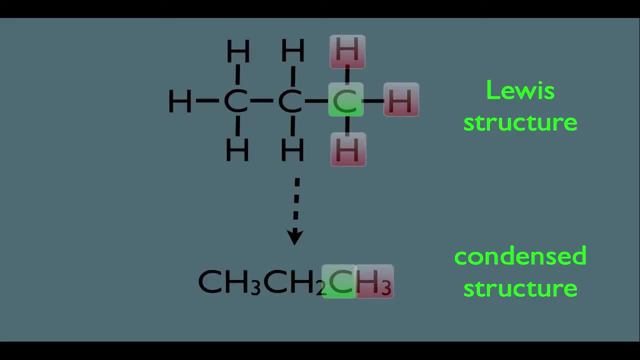 three hydrogens here are collapsed down to these three hydrogens here. And while we're looking at this molecule, I'd like you to also know that it's what's called an alkane. An alkane is a molecule that has only carbon in it. 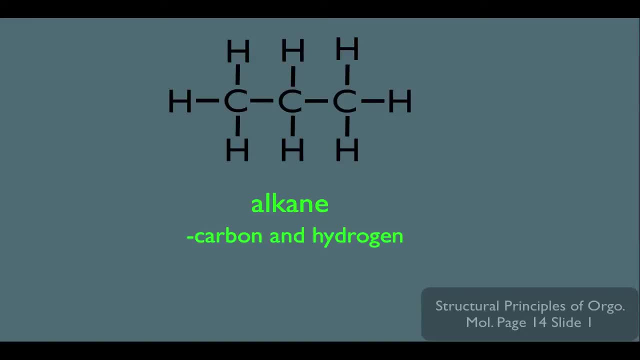 It includes carbon and hydrogen, sometimes called hydrocarbons, And all of the carbons in the molecule are sp3 hybridized. Now that we got this down, let's use alkanes to help us better understand intermolecular forces and how. 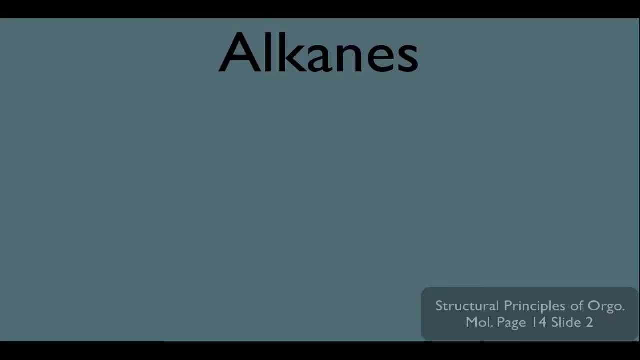 they dictate physical properties of organic molecules. And here's one of the things I want you to know: the relationship between molecular weight, boiling point and melting point of加 alkanes. here it is: The higher the molecular weight, the higher the boiling point, and 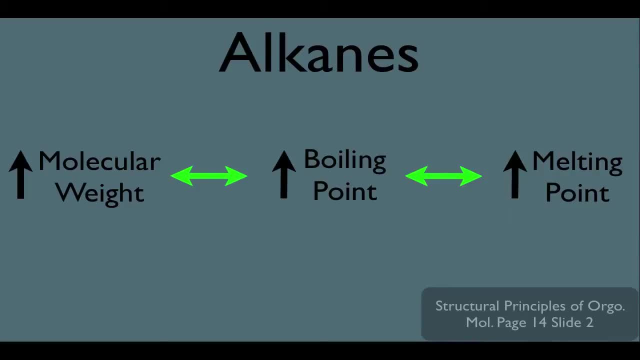 also the higher the melting point. We need to remember this about alkanes, But we should also understand why this is the case. But before we go into the why, I just want to quickly show you one more way to represent organic molecules Again. 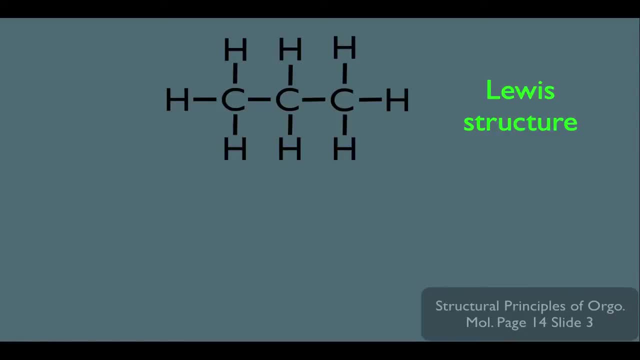 remember. this is our Lewis structure To help me better explain the principles in this lecture. we're going to want to think about this molecule as this representation. This is called the bond-line formula And here's how we interpret it: These three carbons right. here would be these three points, right. 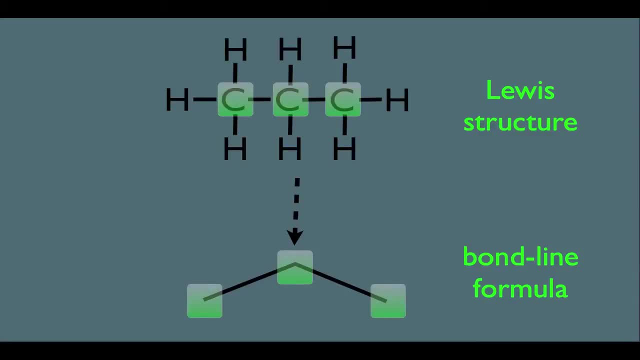 here. So here's how you could think about this bond-line formula representation. It's just a trace of the carbons within an alkane And notice, we're not showing any of the hydrogens. The name of this compound happens to be propane. We'll go. 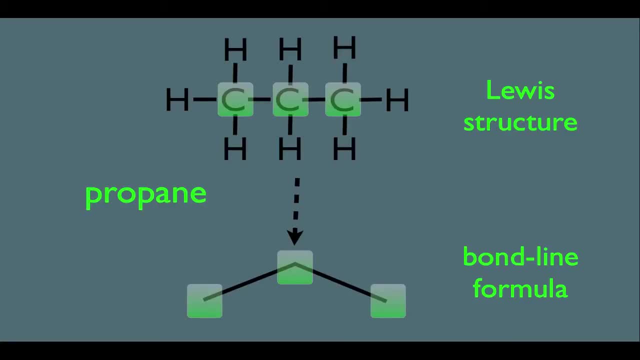 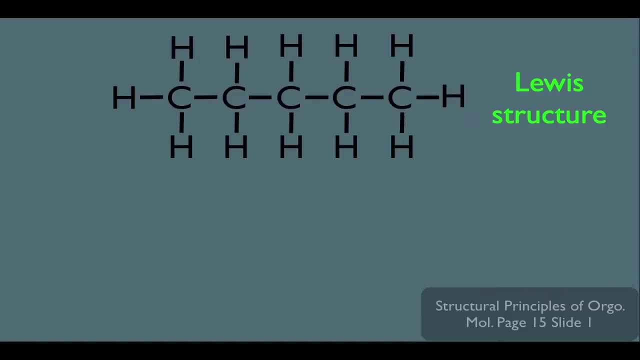 into more detail on that later, But to just make sure you got this, I'm also going to talk about this molecule right here. This is his Lewis dot structure And this right here would be his bond-line formula. And again, the five carbons here in this chain would be these: 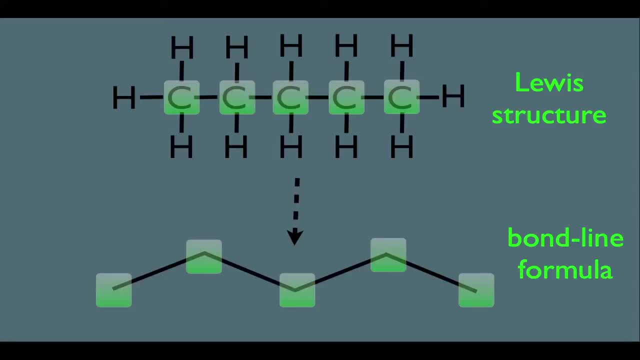 five points down here. The name of this compound happens to be pentane. So again, in this representation we really only care about the length of the carbon chain of the molecule. So let's look at an example here. Let's say I have two molecules, one each, in a. 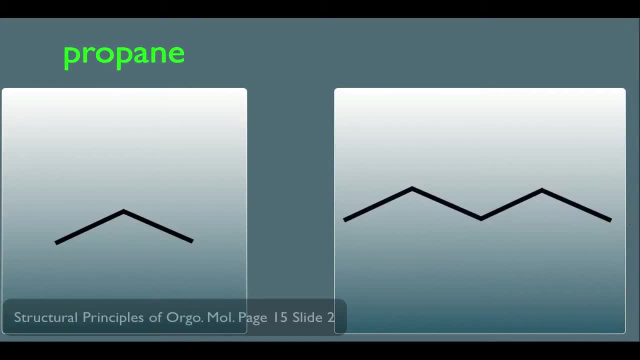 beaker. I have propane over here and I have pentane over here on the right. Let's see why one of these would have a higher boiling point than the other. So let's look at the propane first. Remember we don't have just one propane. 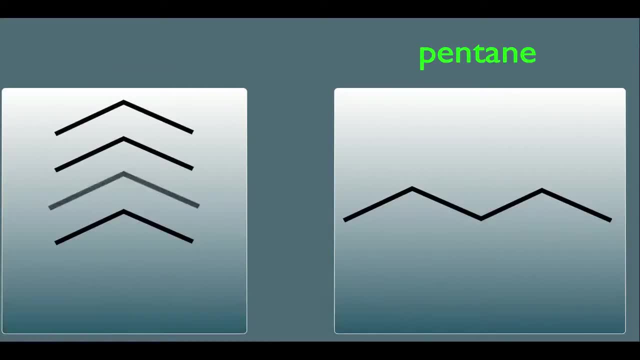 molecule in the beaker. We have many propane molecules like this, And what's happening here is that these propane molecules are being held together by what's called intermolecular forces. In general chemistry we learned about these And these type of intermolecular forces happen to be called induced dipole. 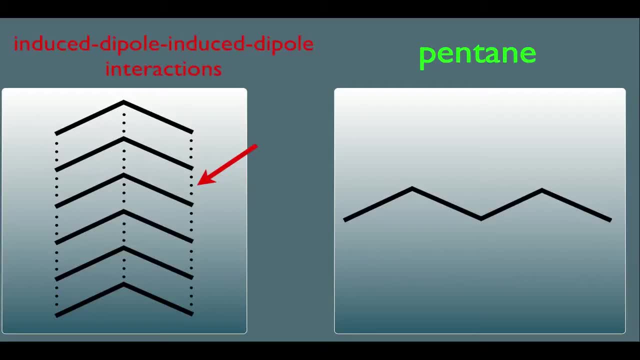 induced dipole interactions, Or you can call them van der Waals forces And even another name: some textbooks refer to them as London dispersion forces. It's these forces that keep all the propanes held together in a liquid form, And in order to get propane to evaporate, you would need to 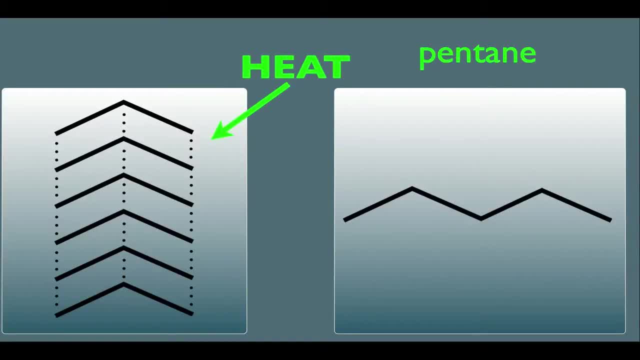 add heat, And heat would need to break these intermolecular force bonds right here, enabling the propane to evaporate out of the solution as a gas. If that's the case now let's analyze pentane the same way. Again, these would represent the 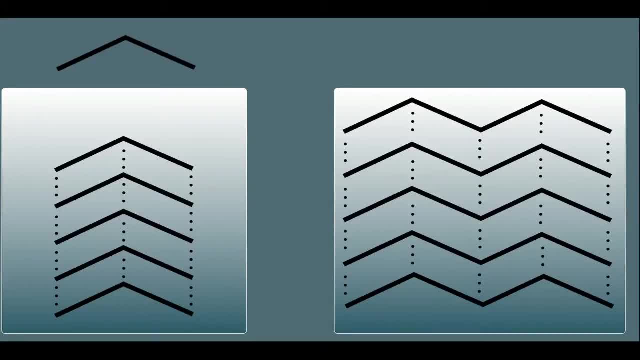 intermolecular forces. Notice: compared to propane, pentane has a greater number of intermolecular forces per molecule. So that means to evaporate pentane adding the heat we'd have to break more intermolecular force bonds to get him to evaporate. Pentane is going to 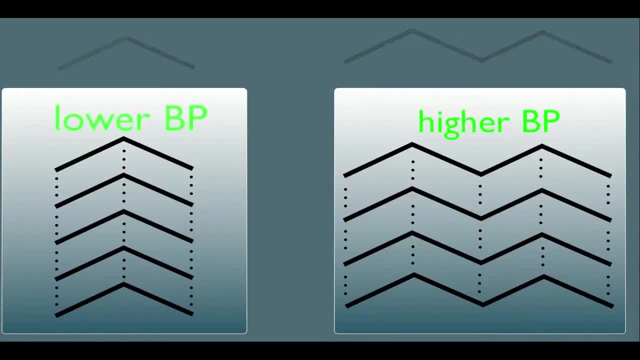 have a higher boiling point and propane is going to have a lower boiling point. It simply takes more energy to separate the pentane molecules than it does to separate the propane molecules, And higher energy therefore means a higher boiling point. So that explains that trend there. 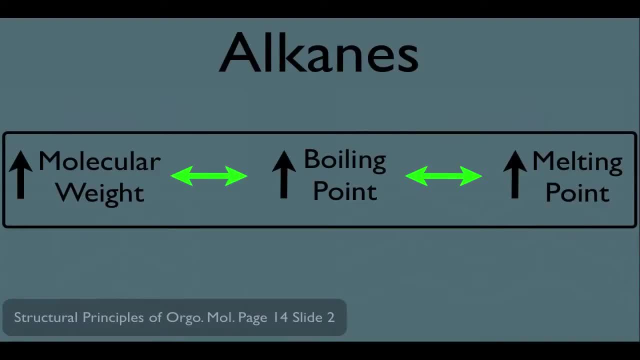 That's why an increased molecular weight corresponds to a higher boiling point, And what we saw also can be applied to melting point. Again, the higher the molecular weight, the higher the melting point. for the same reasons, The more intermolecular forces you have, the higher temperature it takes to melt something. 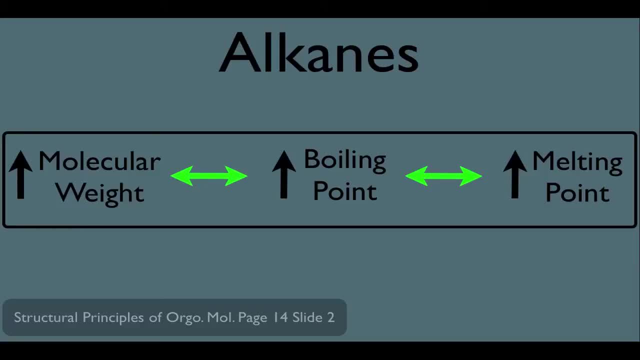 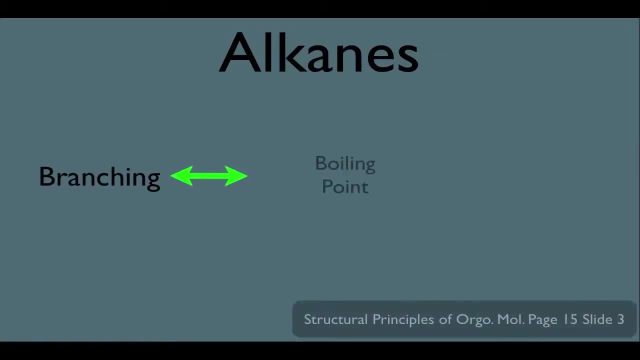 But there's another relationship between the structure of an alkane and its boiling point, And I'd like you to know that, And that's basically this right here: Branching, How does that affect boiling point? Well, what I'd like you to know is that more branching. 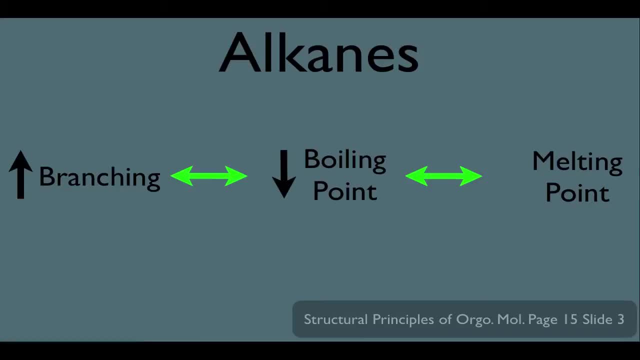 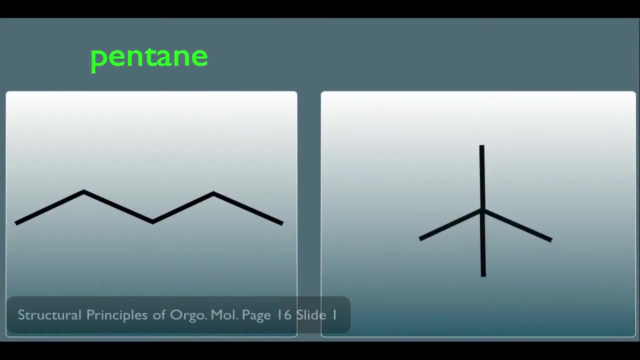 causes a lower boiling point but increases the melting point. We also want to remember this trend And let's understand this one as well. Let's say again: I have two samples: here I have straight chain pentane And in another beaker I have 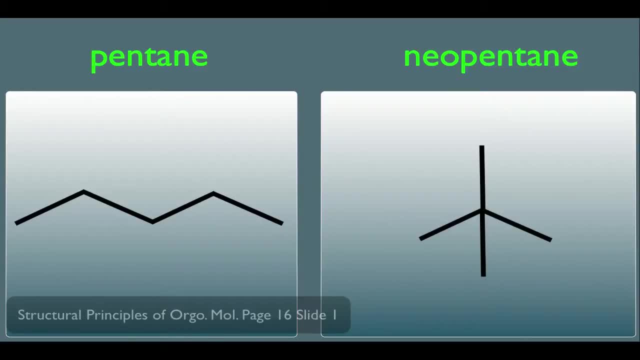 neopentane. Neopentane is just the common name for this molecule. Notice, it happens to have five carbons. That's why it's a pentane And it's very branched. So let's look at the analysis here. In the left beaker of pentane, remember, we have a 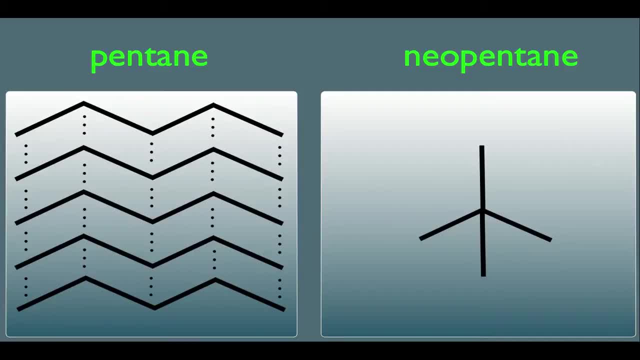 bunch of it here And they're all connected by their intermolecular forces. And remember, in order to evaporate or boil off pentane, we need to add heat. Heat needs to go in and break all of these intermolecular force bonds here. Now let's do the same analysis to neopentane. 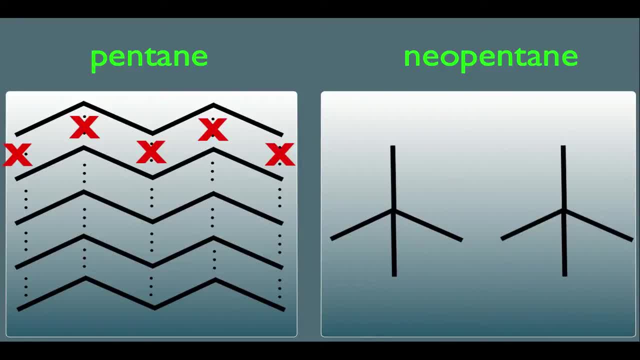 Let's say we have more than one here in our beaker And notice, because of his branching there's going to be less overlap of the molecules. therefore there's going to be less number of intermolecular forces to connect these two molecules. In this case we see only one. 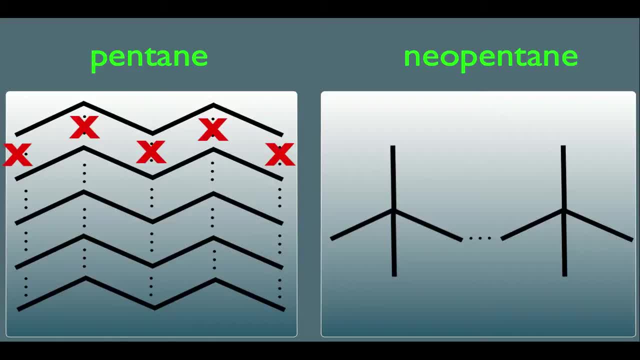 So that means, in order to boil or evaporate neopentane, you add heat and therefore need to break less intermolecular force bonds. So that's the effect of increased branching. This means that straight-chain pentane is going to have a higher boiling point and 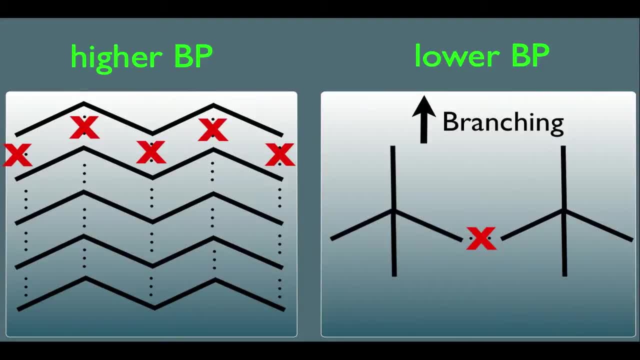 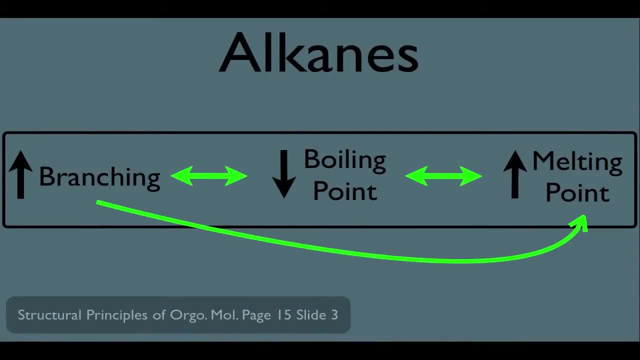 neopentane is going to have a lower boiling point. Now let's go back to our trend here. What we're seeing here is increased branching corresponds to a higher melting point, Even though we just saw it corresponds to a lower boiling point. How do we resolve this? 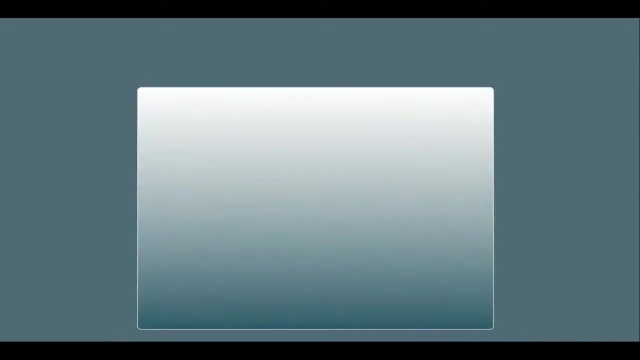 Well, let me show you how this makes sense. Let's say again: we have our neopentane here, a very high branching molecule, in a beaker, and let's place a whole bunch of it in here. Now think about it. Melting point is when you go from. 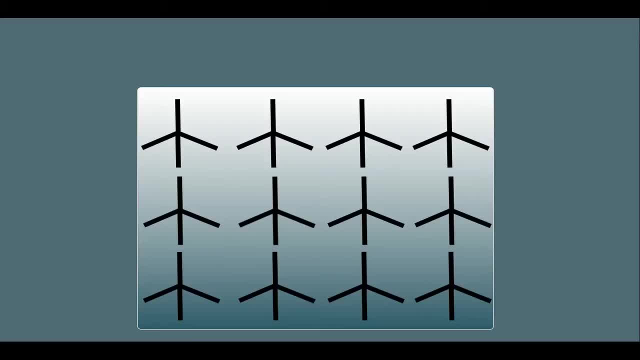 a solid to a liquid, And what I want you to see here is that the more branching you have think about it, the molecule becomes more compact. And the more compact the molecule, the more easy it is to pack them together in a lattice. 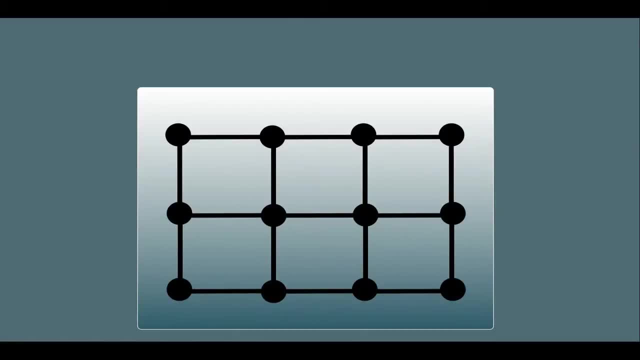 framework such as a solid. This is why increased branching leads to higher melting points. So, basically, the increased branching increases the ability to pack this molecule together, so therefore it takes more energy, a higher melting point to separate these molecules into the liquid phase. 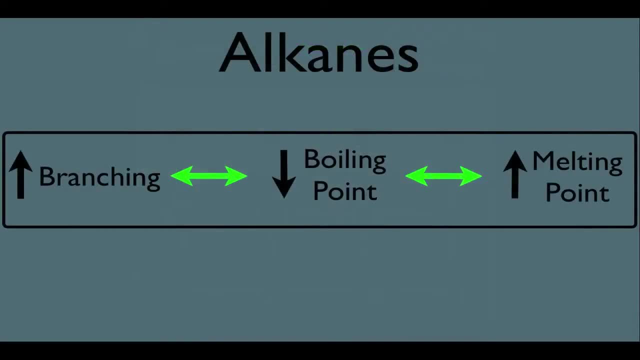 So that's why we observe this particular trend. Another interesting point about melting point and alkanes is that an alkane with an even number of carbons have higher melting points than alkanes with an odd number of carbons, And this is also for the same reason. It just so happens that 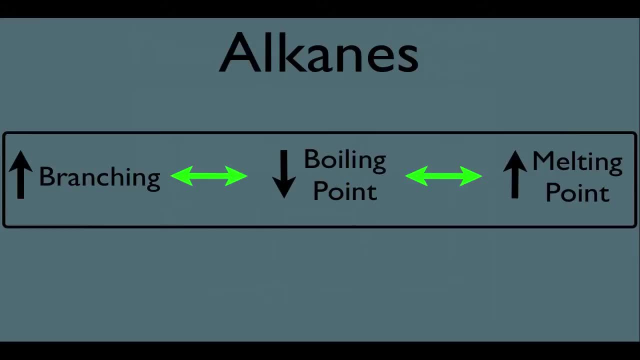 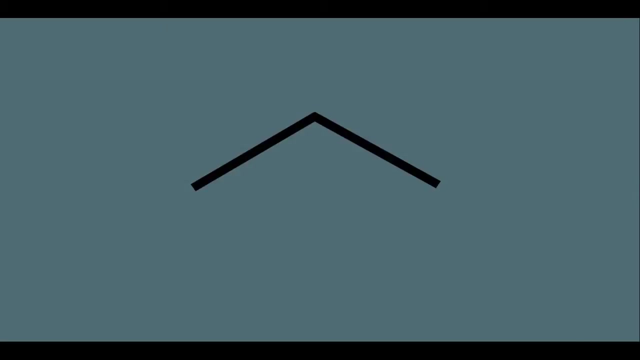 alkanes with an even number of carbons can pack themselves together better than having an odd number of carbons. Now, just to be sure, here let's understand how alkanes could have intermolecular forces in the first place. For instance, let's look at propane right here. 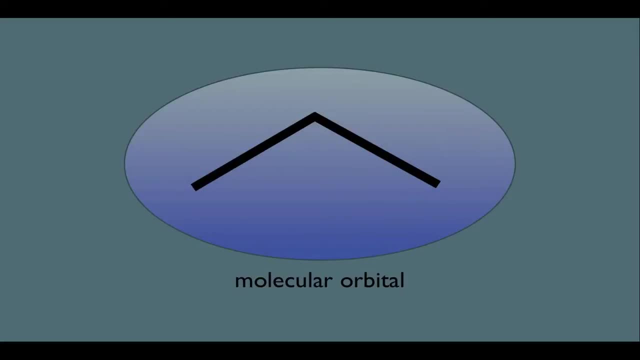 And let's pretend, this happens to be his molecular orbital, which means the electrons around him could be anywhere in this vicinity. Remember, because alkanes are made up of carbon and hydrogen, there's not a big difference in the electronegativity of carbon and hydrogen. 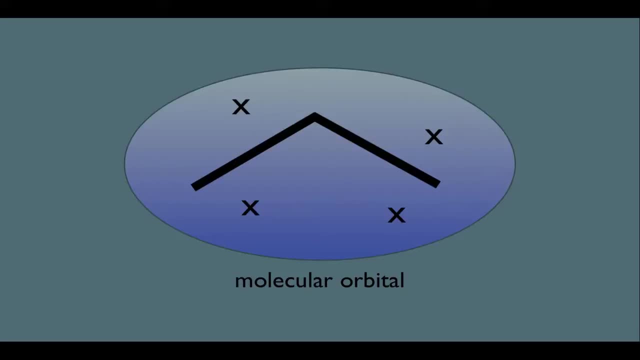 So there's no polarity, no polar bonds in this molecule, which means alkanes shouldn't have a partially positive end and a partially negative end to their molecule. In other words, they shouldn't have a dipole moment. However, what happens when you happen to have a bunch of, let's say, propane in a beaker?